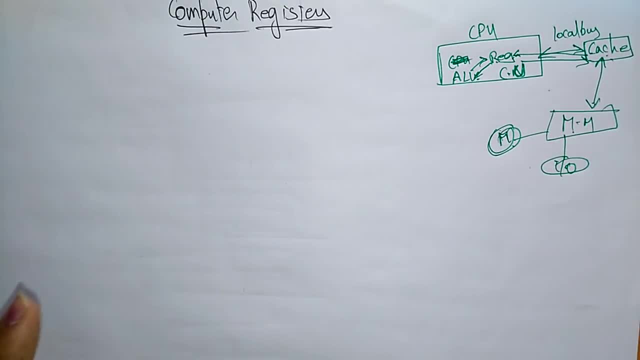 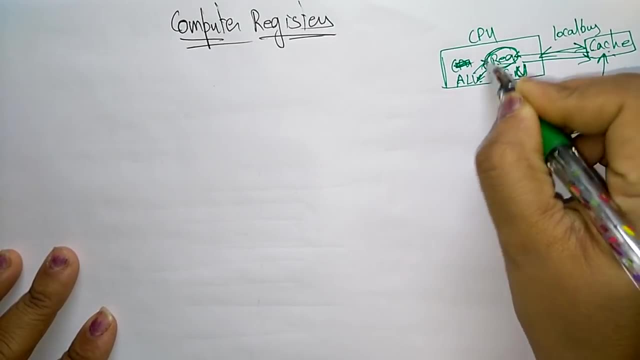 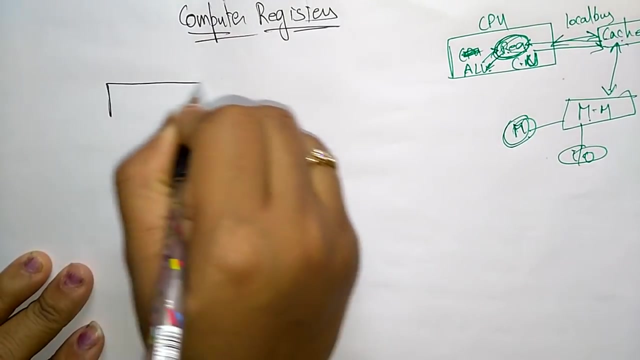 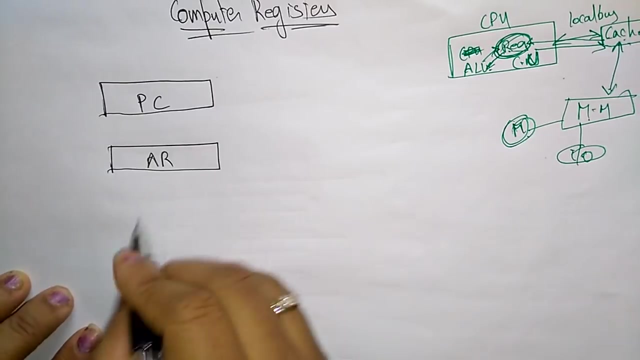 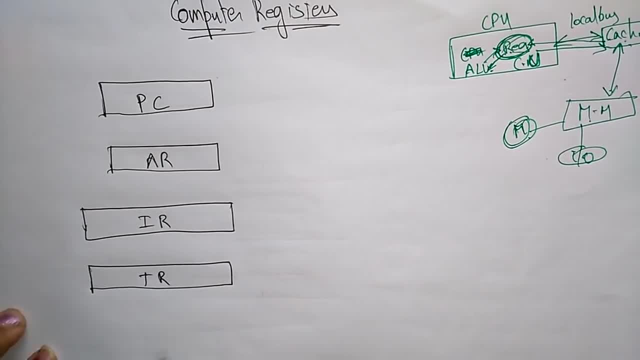 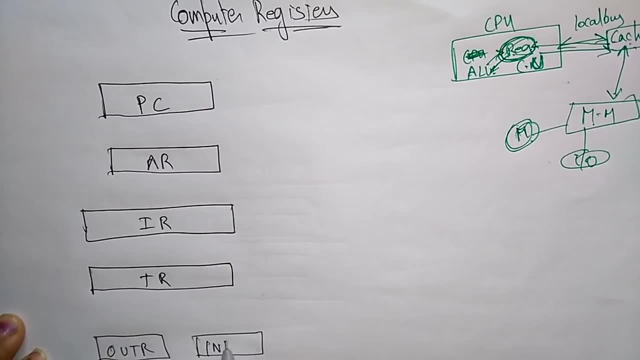 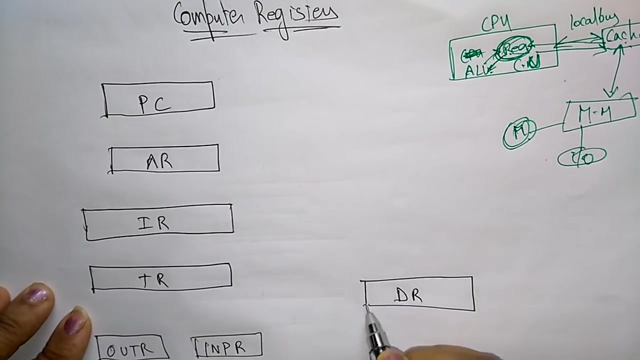 whatever the data that has to be sent from memory input output to main memory, main memory to cache, cache to registers and registers will send to main memory. So temporary register: outer register output register, input register. next data register accumulator. 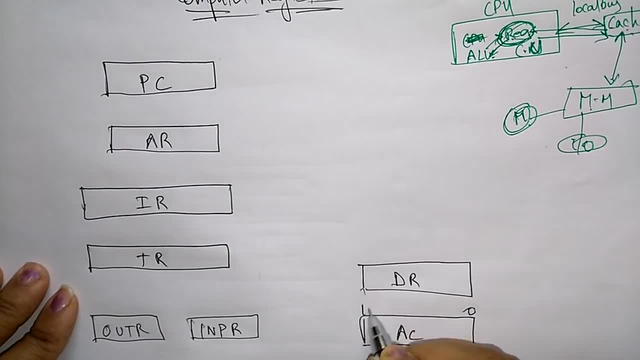 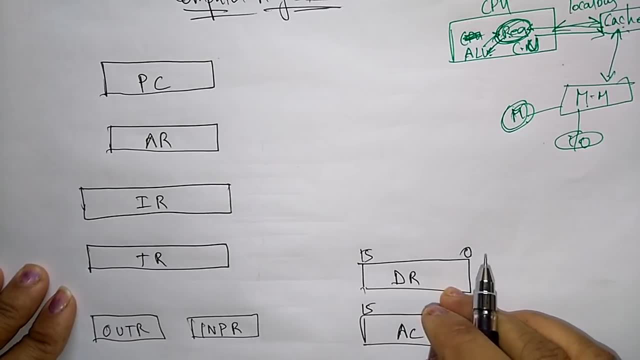 So accumulator stores up to 0 to 15,. 16 bit of data will be stored in accumulator Data register. also 16 bit of data will be stored here. Input register: only 8 bit. output register: 8 bit 0 to 7.. 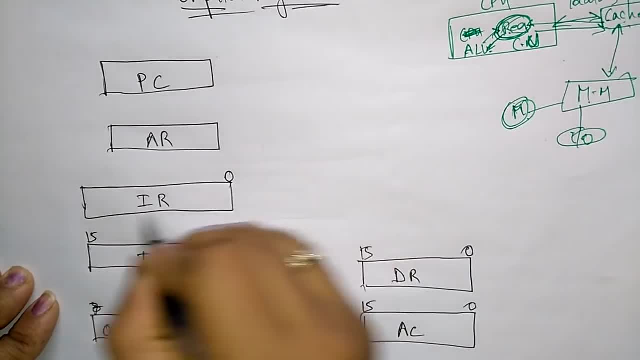 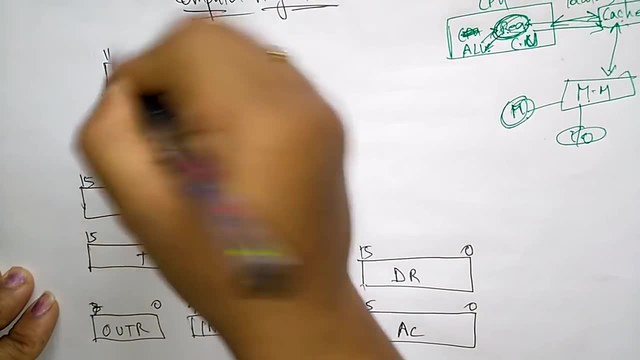 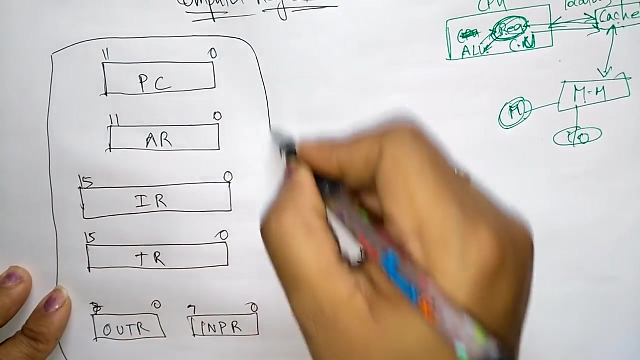 Temporary will hold up 16, it is 16 bit register. Instruction register is also 16 bit, whereas address register is 12 bit. Program counter is also 12 bit. So this is completely you call it. these registers will be present in. 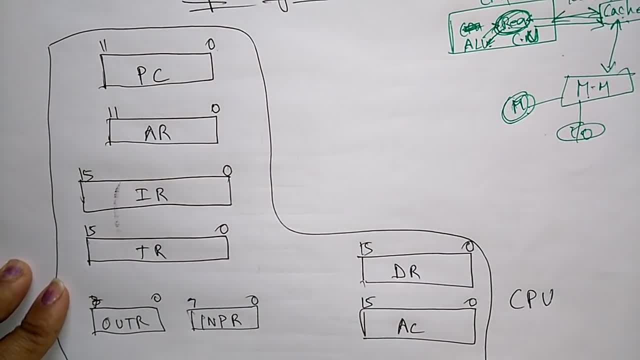 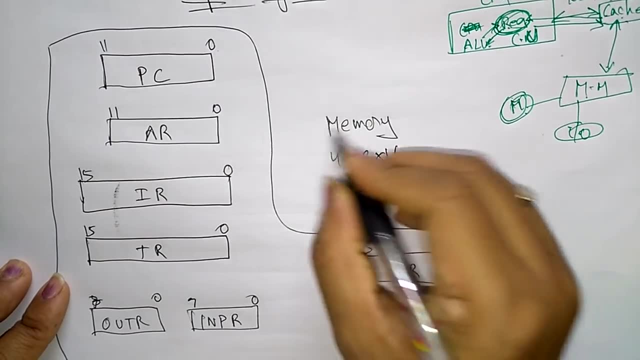 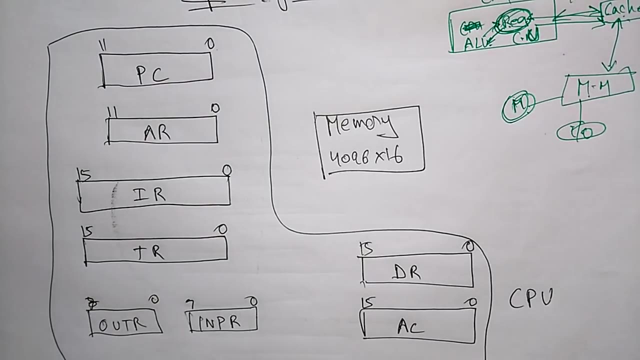 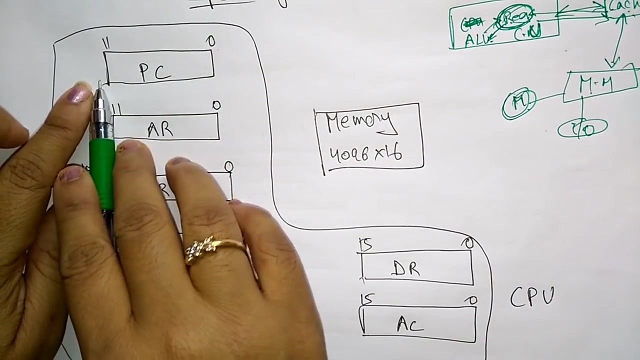 CPU Central Processing Unit. All these registers will be present in Central Processing Unit And here the memory size: 40916 to 16.. So this is the memory size of this CPU. Okay, So here you can observe a program. counter is nothing, but it holds 12 bits, 0 to 12 bits. 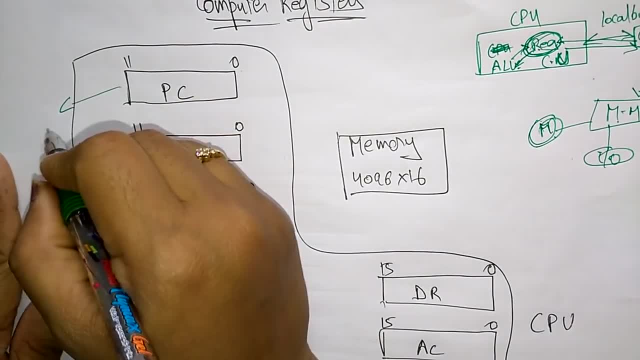 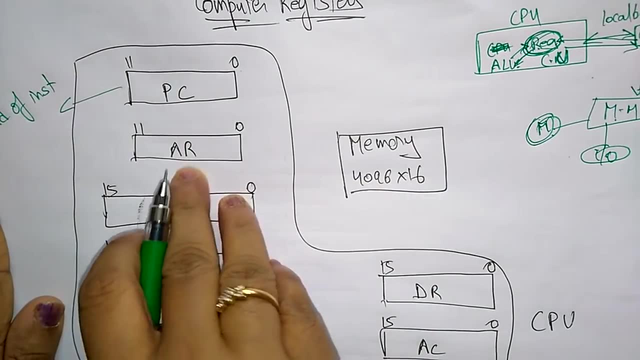 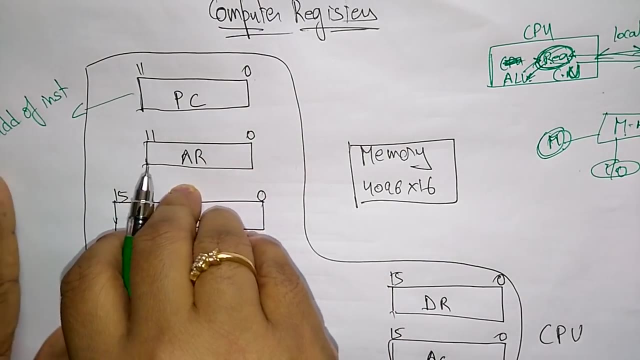 So what it holds, The program counter always holds that Address of the instruction. it holds the address of instruction, Whatever the instruction that has to be executed next. that instruction address will be stored in the program counter, Whereas AR arithmetic register. so this is also a 12 bit register. 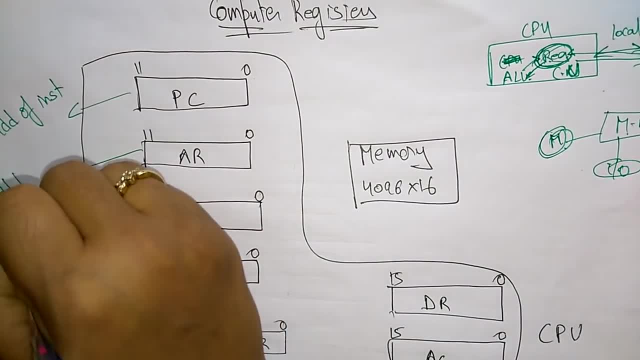 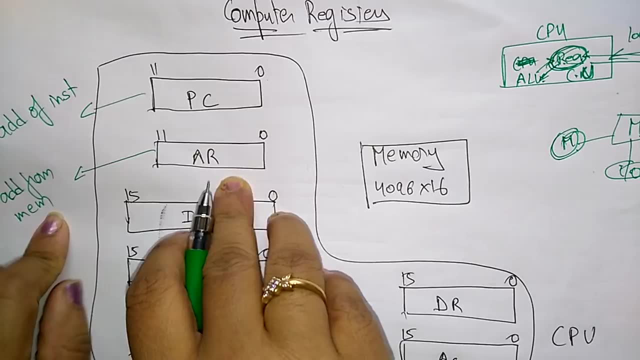 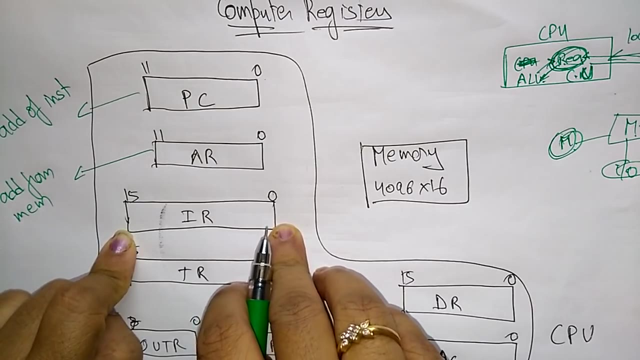 it holds address from memory, address from memory. So whatever the data that you are taking from memory, so that address from memory will be stored in address register. Now coming to IR. IR is nothing but instruction register, So instruction register is a 16 bit register. 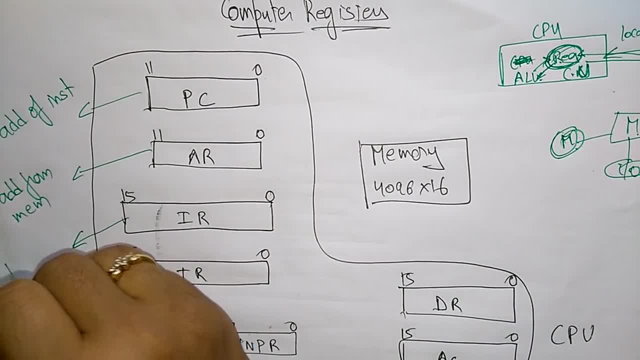 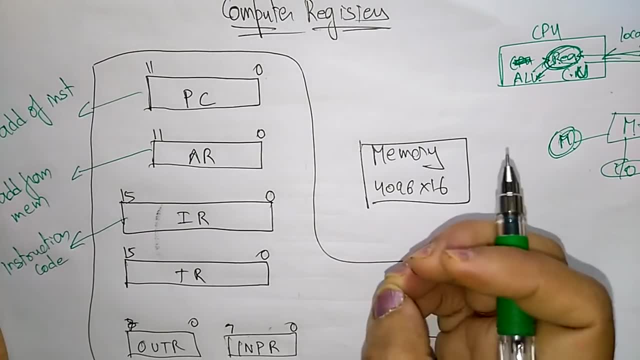 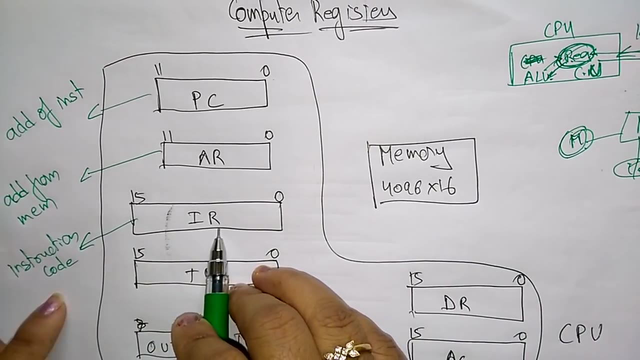 It uses to hold instruction codes. Some codes will be there for each instructions for add, subtraction, increment, decrement, for everything. For opcodes there should be a code So that code will be stored in instruction register Next TR. 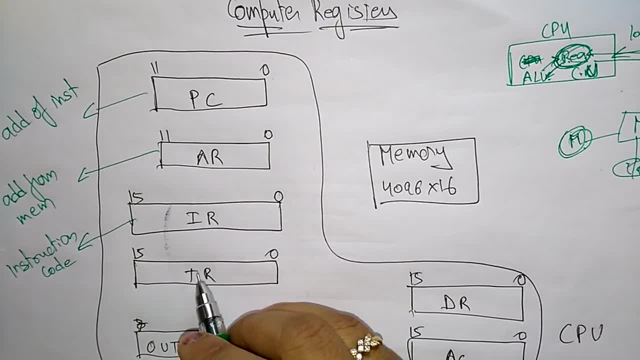 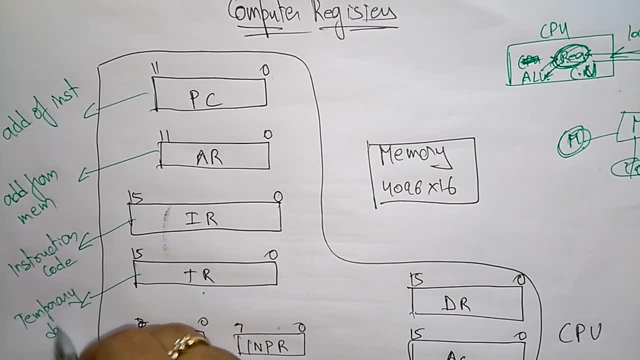 TR is nothing but temperature, So it is a 16 bit register. So it is a 16 bit register and it holds temporary data. Okay, And outer OUTR is 8 bit and INPR is an 8 bit. 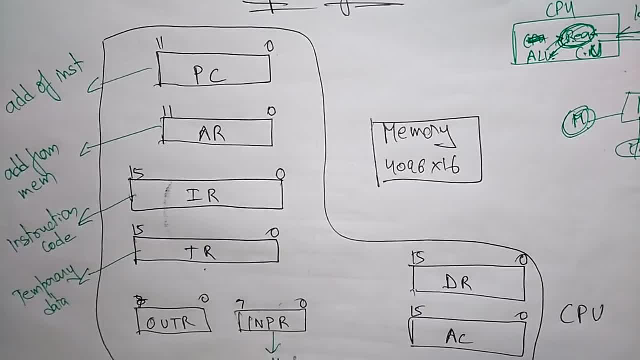 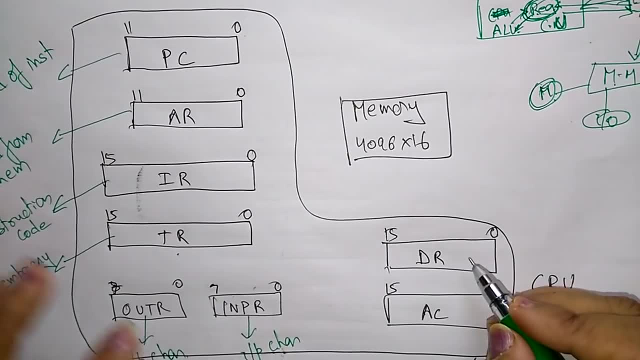 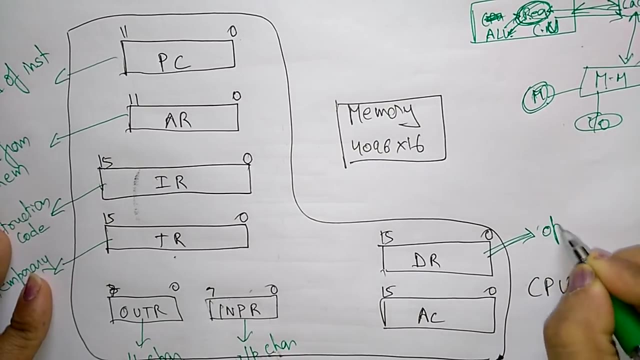 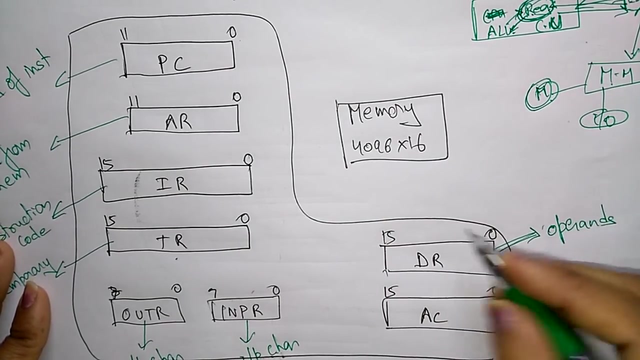 So INPR holds input characters, Whereas out here holds output characters. Now coming to DR. DR is nothing but 16 bit register. It holds the operands. holds operands means the data that is stored in a variables- Those you call it as operands- and accumulator is used to store the result. 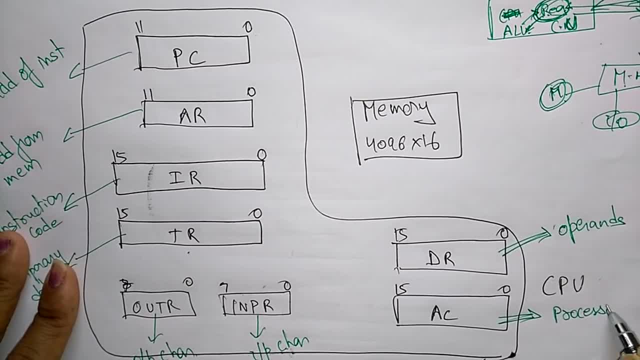 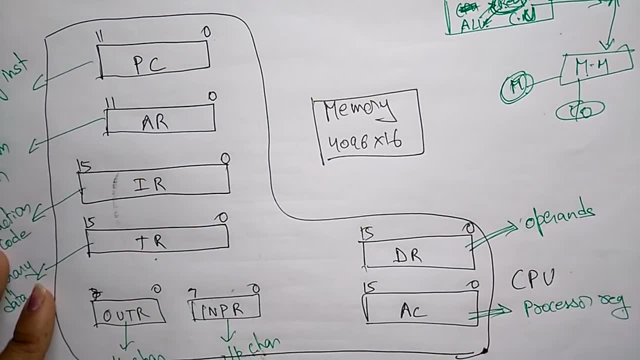 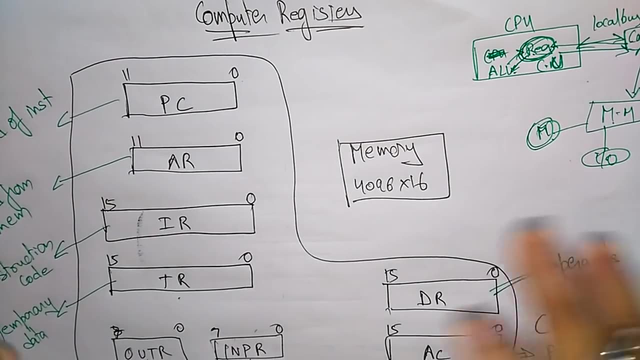 You call it as a processor register. processor register- The name for accumulator is a processor register- means it holds the result of an operation that will be stored in accumulator. It is a 16 bit register. So these are the different registers that are used in the central processing unit. 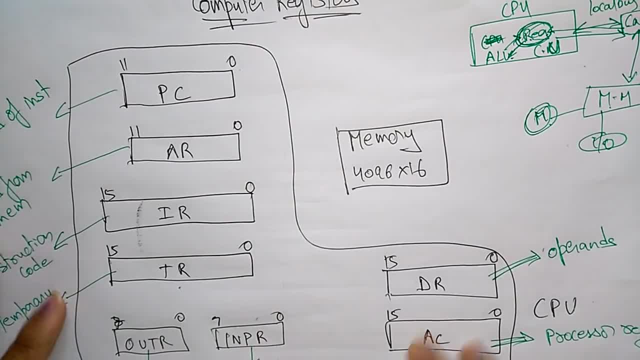 So each performs their own operation to perform the calculations. So this is about the computer registers. Thank you.